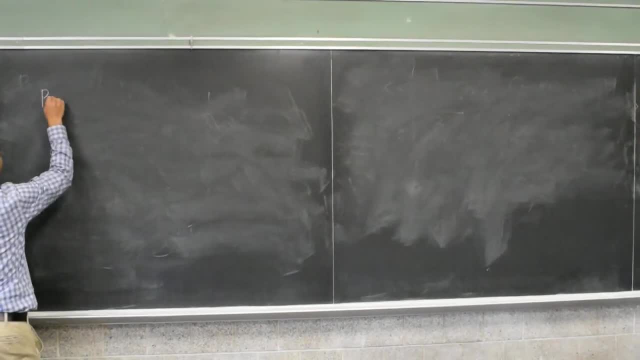 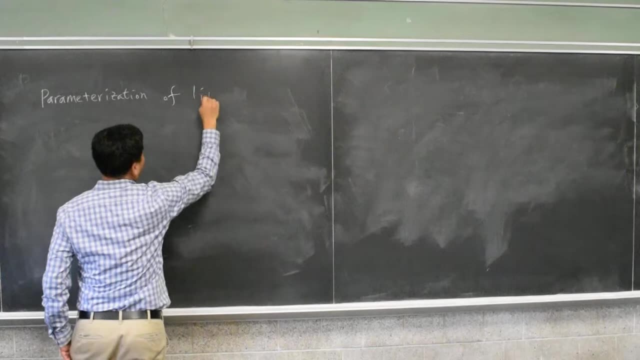 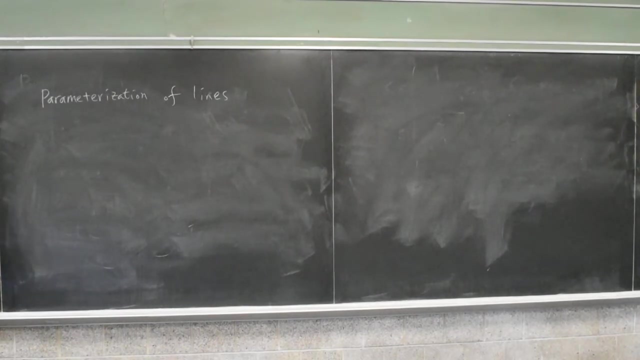 Now sometimes, instead of giving a formula to parametrize, you're just given the curve and you have to parametrize it. So suppose you have 1 comma 2, and say you get 3 comma negative 2, and I want a parametrization of that line connecting the two points. 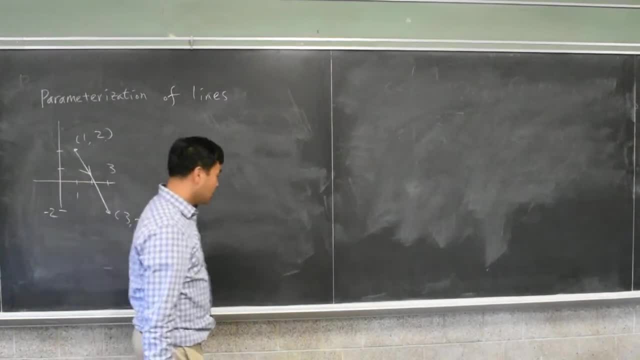 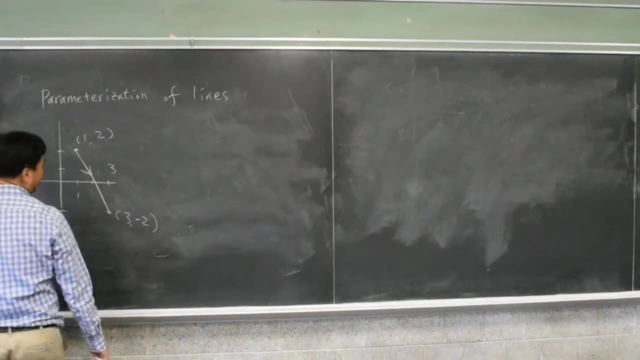 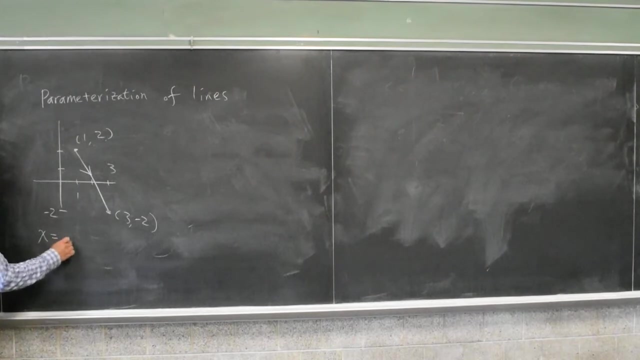 How do you do that? Well, the easy way is to think about the parametrized form of the line equation and use the direction vector and the point it passes. So what's the parametrized form of the line equation? It's x equal to at plus x0.. 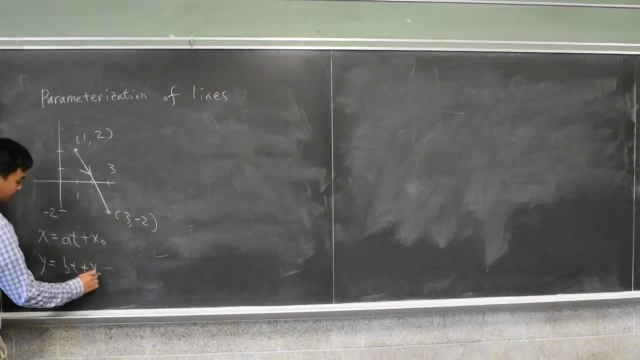 And y is equal to bt plus y, And then a comma b is the direction vector. The vector's direction is this way. so you should determine y as initial to get the direction vector And x0, y0, I usually would state that x0, y0 is any point on the curve. 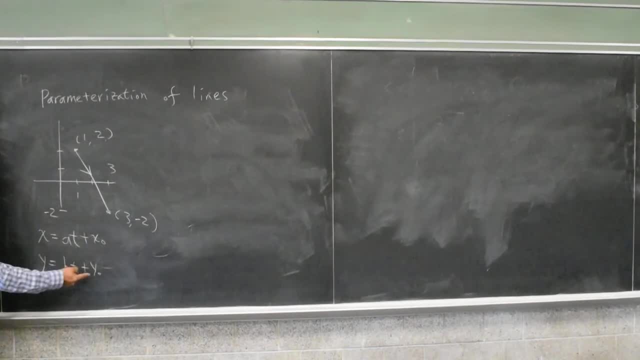 But in this context you should really have it as the point where t is equal to 0. So the beginning point should be x0, y0.. The reason for that is since you're trying to parametrizate only this part. 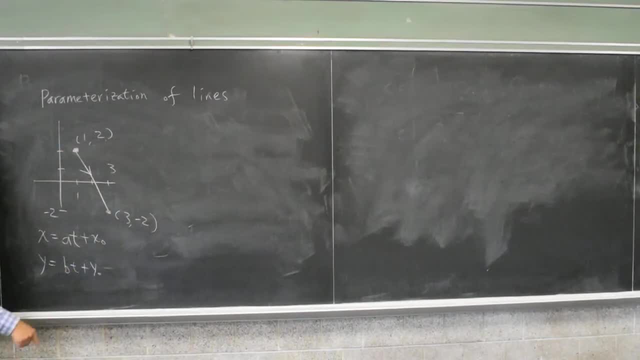 of the line, not the infinite line. if it was the infinite line, you don't care, But if you want only the part of the line, you really want the t equal to 0 to match with x0, y0.. All right, so let's try that. 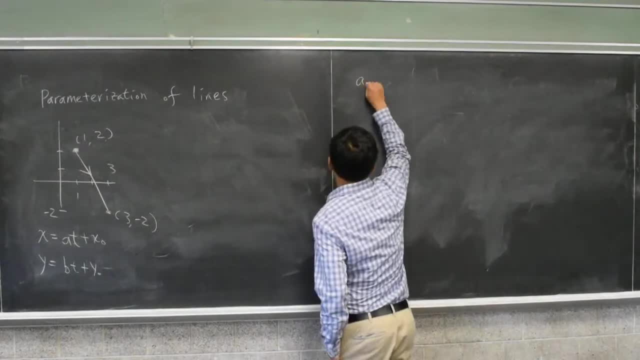 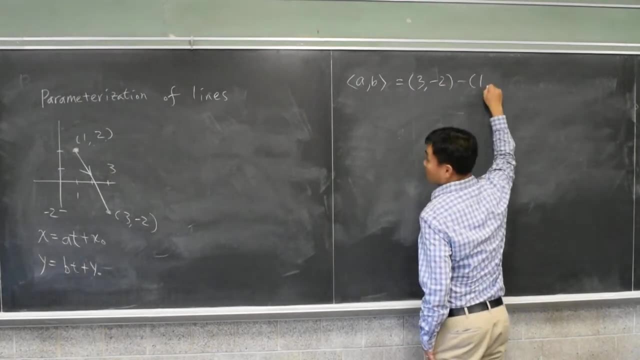 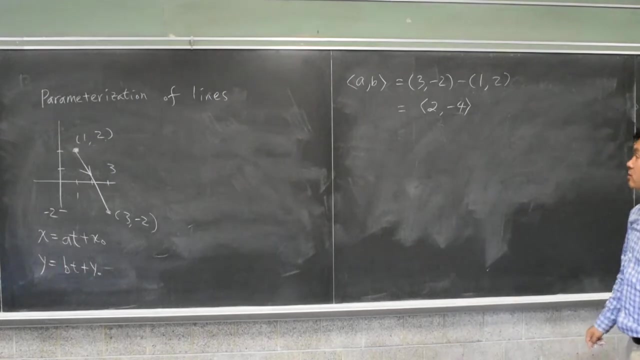 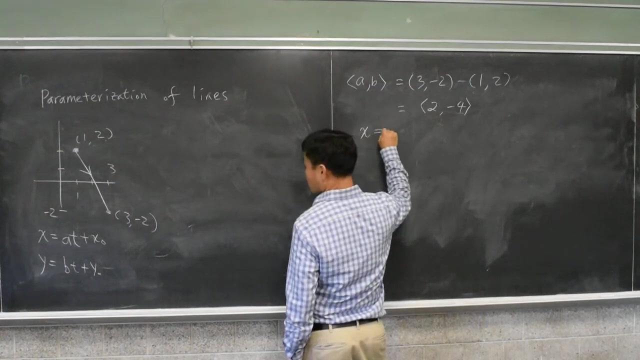 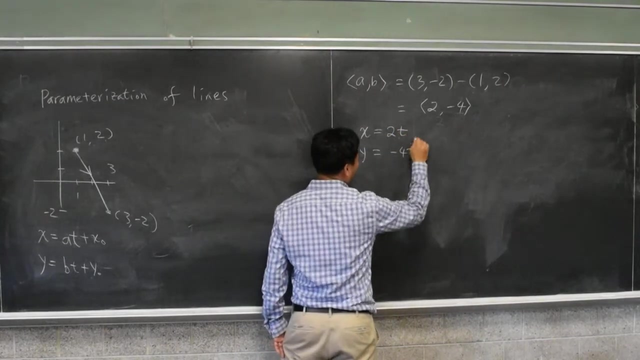 First to get the a b. what do you do You do to get the direction vector? you do terminal minus initial, Terminal minus initial. That's the vector 2 comma negative 4.. And then you can write down your equation as: 2t, y is negative, 4t plus plus, what's? 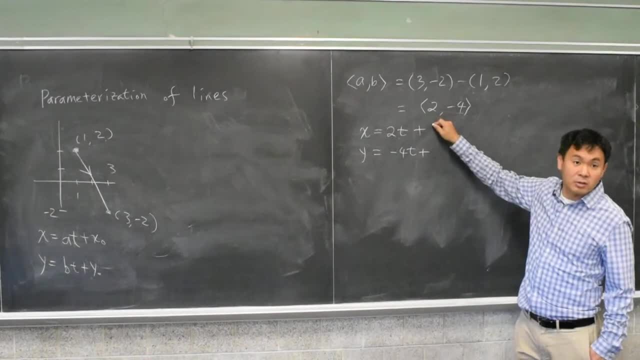 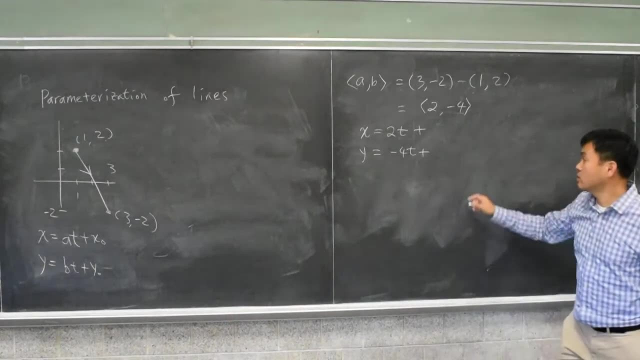 x0, y0?. What should I take for x0, y0?? 0. 0. 0.. 0. 32. 0. 0.. You're just making up numbers, aren't you? 1, 2.. 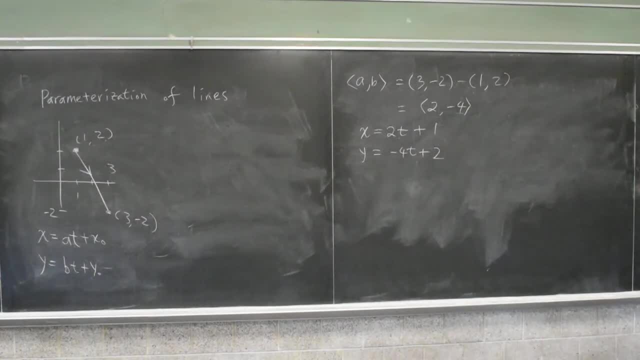 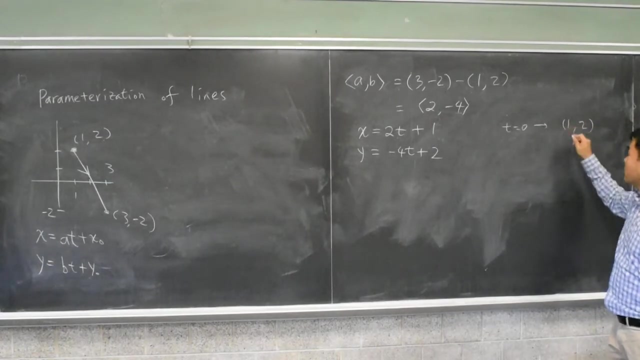 1, 2.. 1, 2.. If you've been listening, it should be easy. OK, All right. so you have this All right, and you do see that when t is 0, the point is at 1, 2,, as you expected. 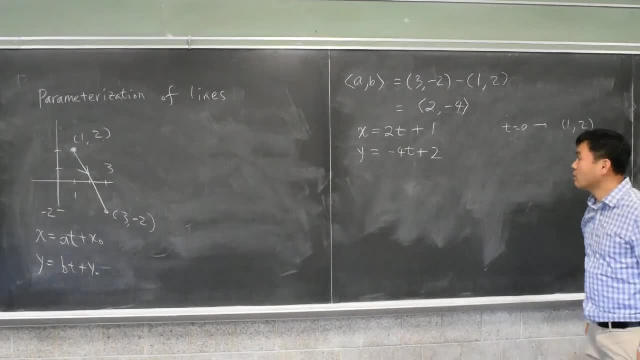 When do you reach 3 comma negative 2? 2.. So for t equal to 1,, you end up with 3 comma negative 2.. 1. 1, OK, Oh, I'm sorry, So you plug in 1.. 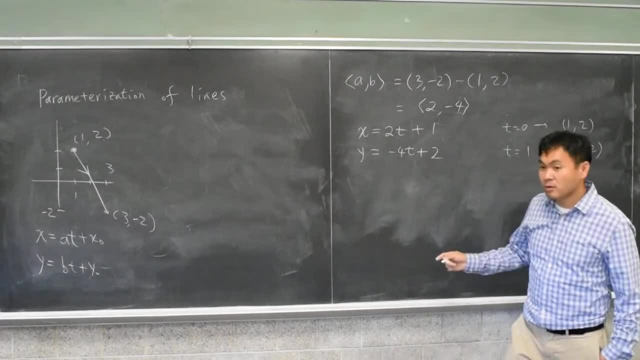 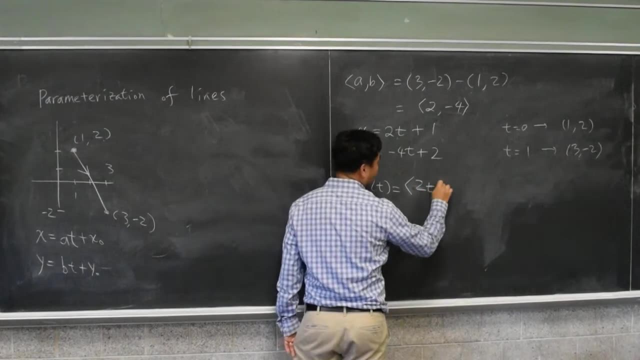 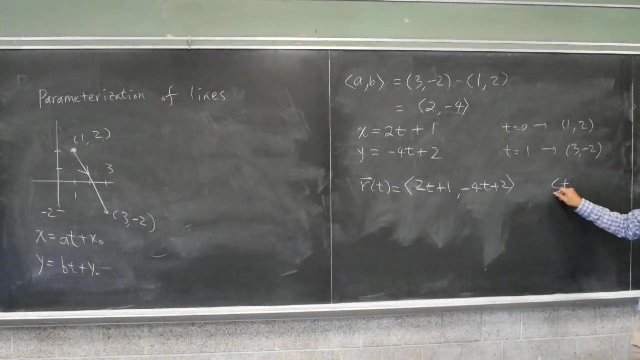 Yeah, if you plug in 1, you get 3 comma negative 2.. So the parametrization is: RT equal to 2t plus 1, negative 4t plus 2, with t value between 0 to 1.. And this goes by for most segments. 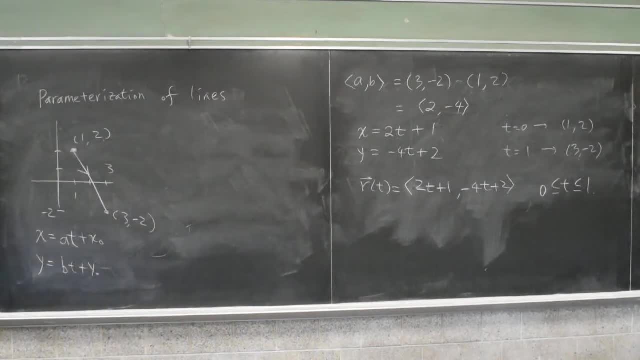 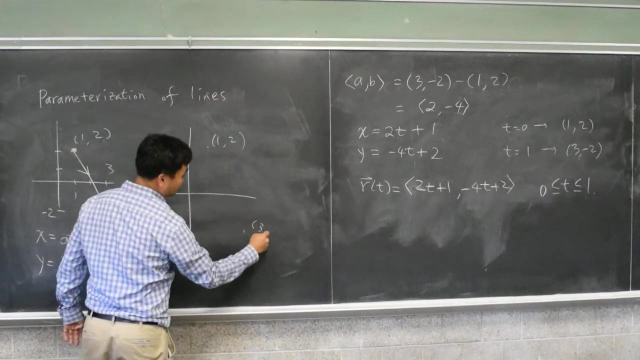 So if you're given any directed segment and you're to parametrize it, you just do the same exact procedure If it was the exact same thing. so 1,, 2, and then 3, negative 2,. if it was the exact same thing but the opposite orientation. 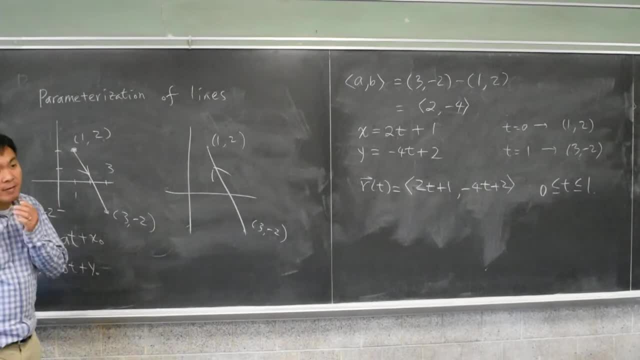 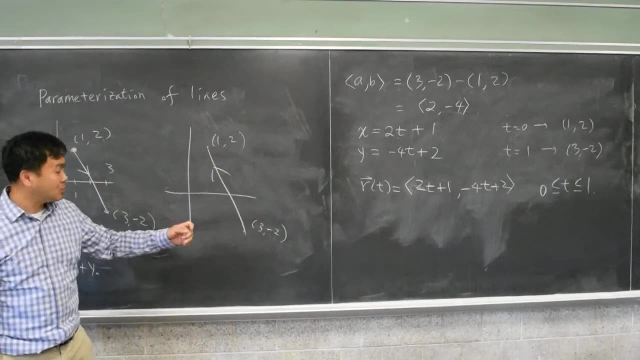 what would you do? You'll be 1 comma 2 minus 3 comma, negative 2.. And your x0, y0 would be taken as 3 and negative 2.. Your t value would still go from 0 to 1.. 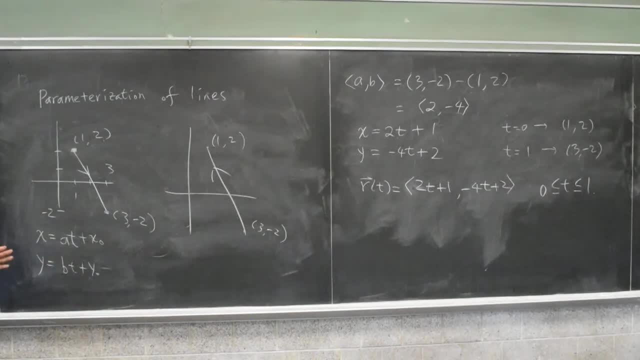 That will give you the exact same segment, but parametrized in the opposite orientation. OK,